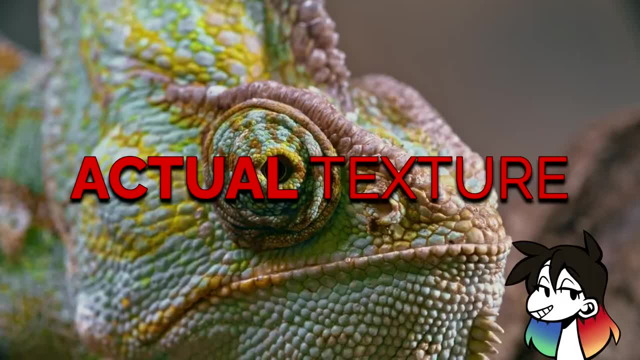 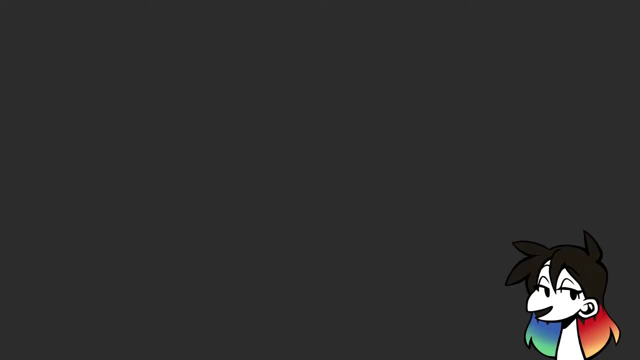 called literal texture, and it's the texture in an art piece that is physically there. There are a few ways to get actual texture. One is by using the actual physical material that relates to what was drawn. For instance, if you illustrated denim shorts, you would use actual. 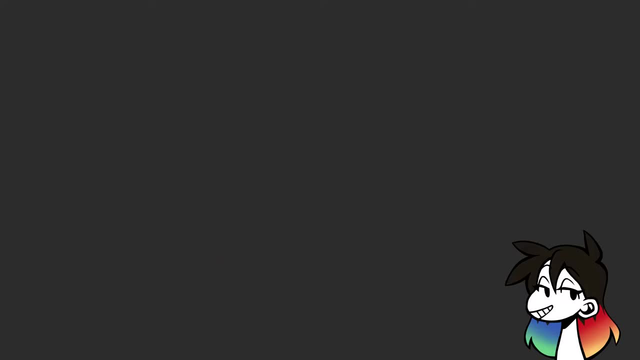 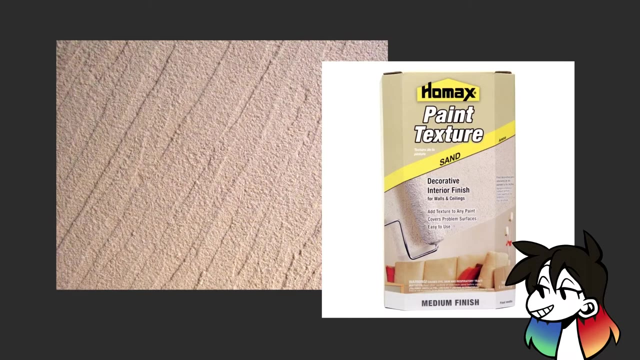 denim as the texture. Another way of showing actual texture is by using the actual physical material. Some artists like to mix sand into their paint to give it a grainy texture. Or perhaps you're using something a little more abstract, like eggshells or stoats, and that will give it an 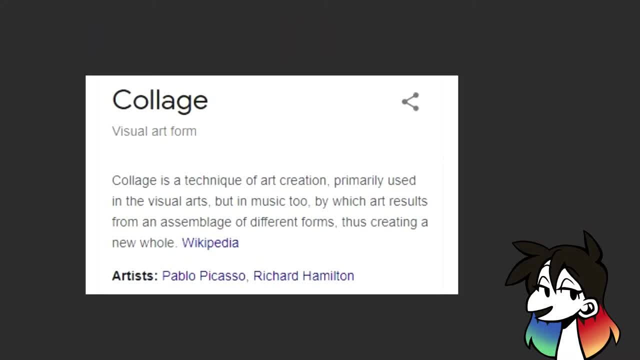 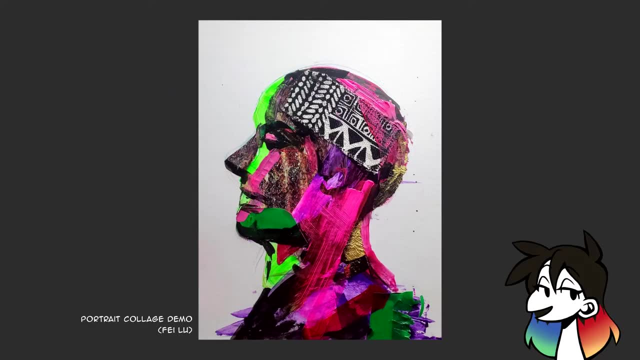 actual texture as well. You can also use a technique called collage, where you use mixed media to create art that has many different actual textures. You could use different fabrics- plastics, papers, clays, garbage- you name it- But the most popular way to give a piece texture is 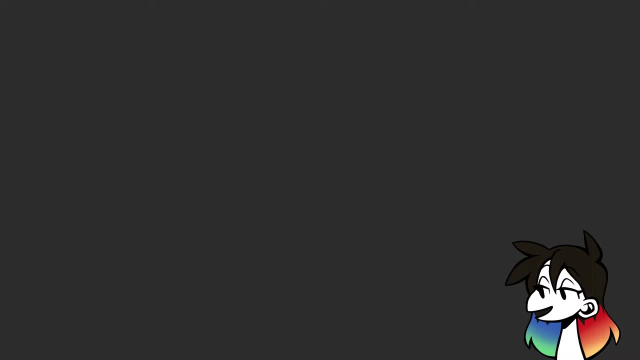 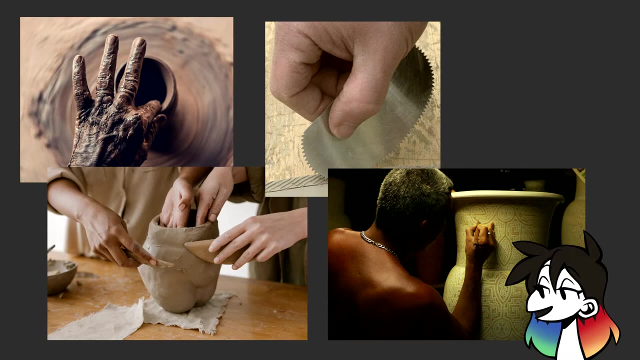 with the techniques and tools used with the medium When it comes to 3D art. there's pinching, pressing, scoring, scraping and so much more. Using a variety of textures. you can create a variety of different textures with your mediums can give actual texture to your pieces When it 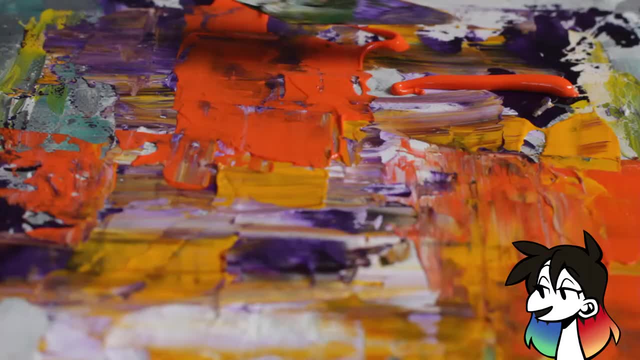 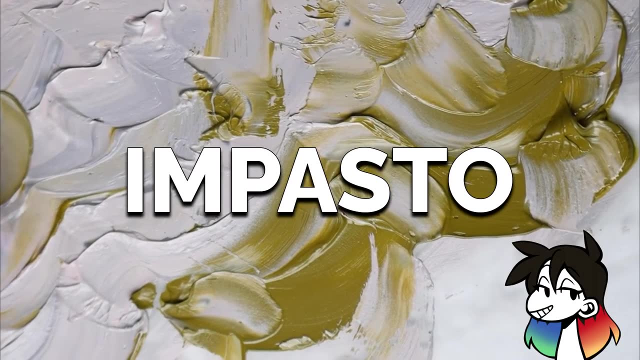 comes to 2D artwork, actual texture is usually done with paint. Oil and acrylic paint can be layered in globs and will dry as a glob, giving it a literal texture. This technique is called impasto, first created in the 17th century by Diego Velasquez, Franz, Hals and Rembrandt. 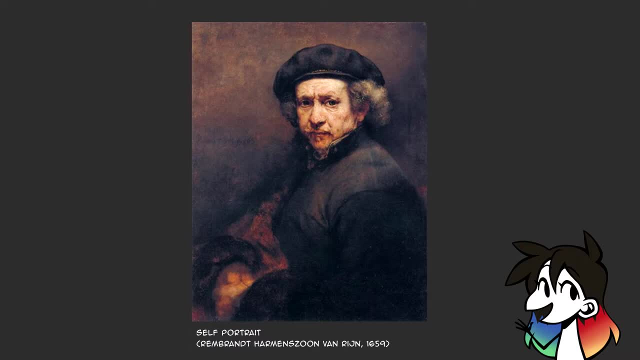 And speaking of Rembrandt, here's his self-portrait painted in 1659.. Obviously, you're just going to have to trust me on this one, but Rembrandt used a lot of impasto to get certain textures on skin and fabric. It's a little hard to see when the image is this. 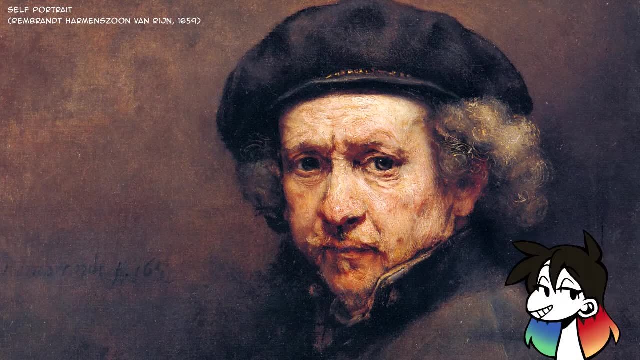 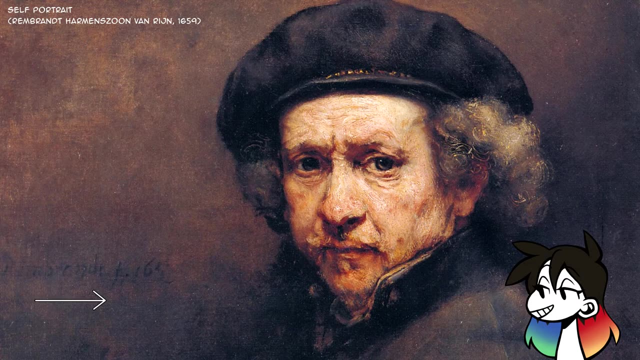 small, so let's zoom in a little here. There we go. You can see all the paint strokes and raised details when you're close up. Rembrandt really liked to use impasto upon the lighter parts of the face and very transparent paint on the background. This adds a really nice contrast. 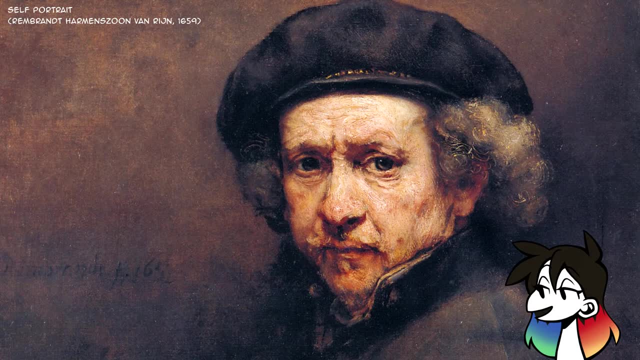 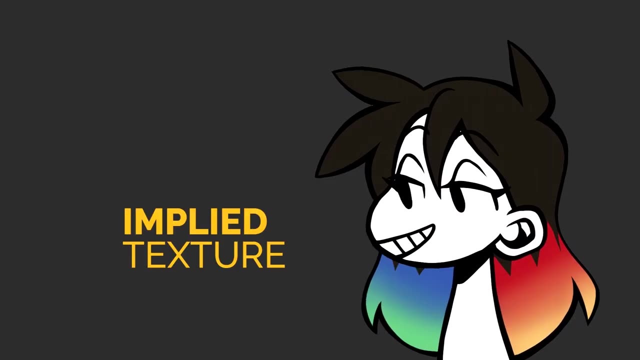 to the piece, which is a principle of design. If you were to touch the canvas, you'd be able to feel all the bumps and textures of thick layers of oil paints. Ironically, because you can't feel it right now, it's more like implied texture. But let me get to the definition of that one first. 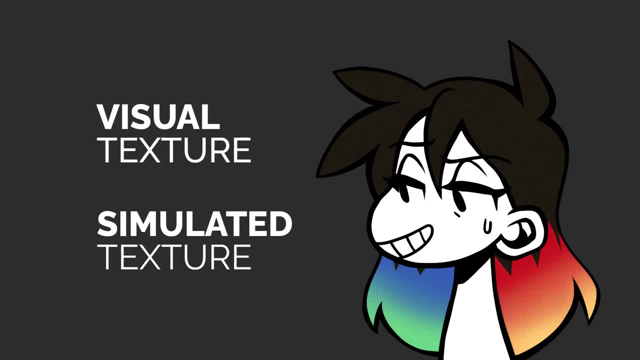 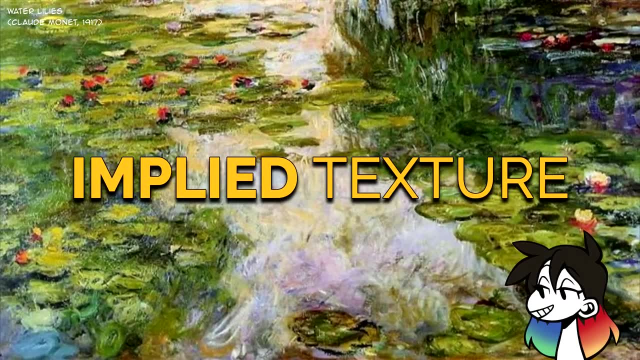 There are so many names for implied texture, like visual texture, simulated texture, so on and so forth, but we'll just stick to implied for this video. Implied texture is texture that isn't actually there, but an illusion, illustrated to look like. 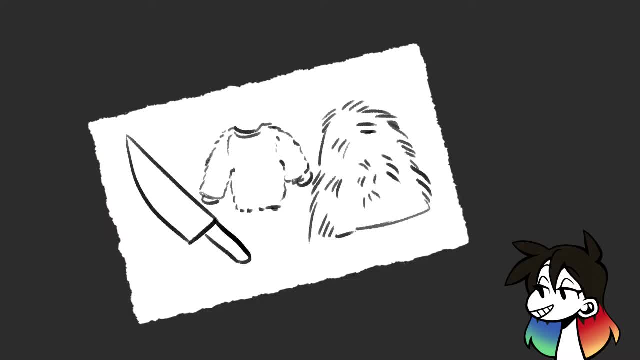 it. This is the one that most of us are used to. Whether someone draws a sharp knife, a fuzzy sweater or a haystack, it'll all feel like a sheet of paper or canvas. You do have a bit of actual texture because of the paper or canvas you'll use, whether the texture quality is matte. 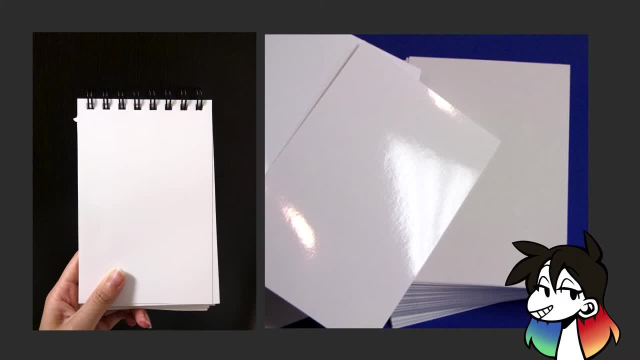 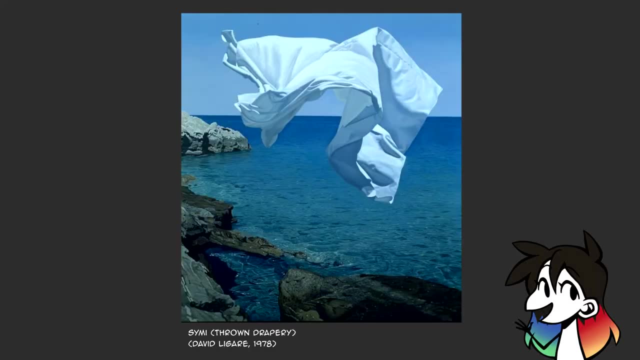 or shiny or whatever, but overall you're just not going to feel the texture that you draw on top of whatever it is that you're drawing on. Honestly, I could use pretty much any piece I wanted for this segment, but to make it look real textury, let me use Simi Throne Drapery by David Lagarre. 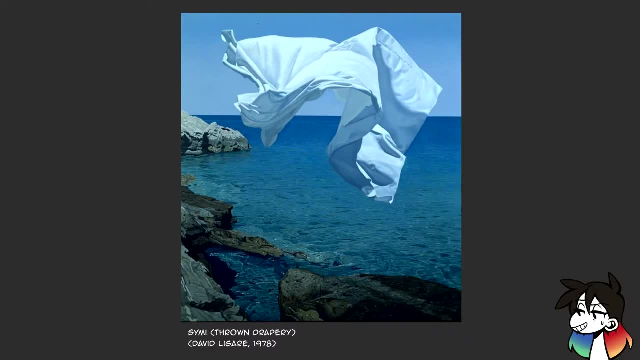 No, this isn't a photo, It's a painting. I know it hurts me a little too with how crazy that is. This painting is done in a style called hyperrealism or photorealism, where the piece looks so realistic that it's almost indistinguishable from a photo. But of course, 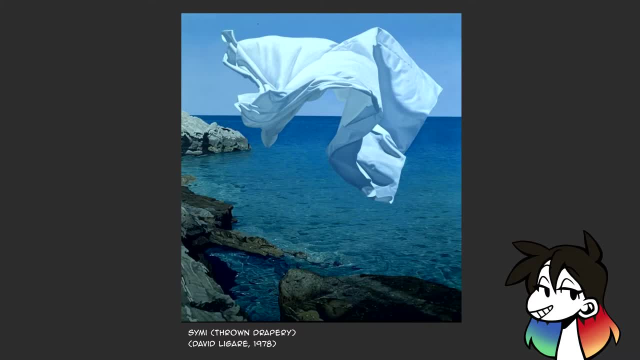 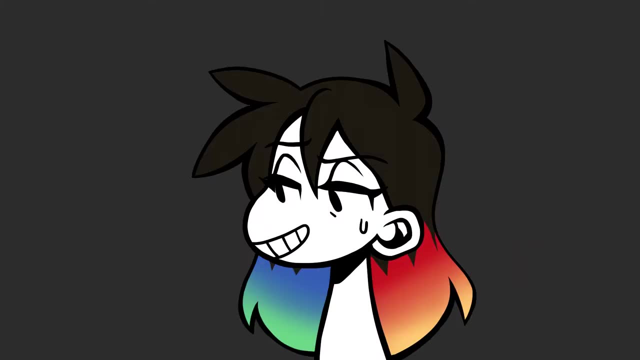 all this texture in the painting is implied texture. You could practically feel the sheet in the wind or the water from the ocean and the rocks on the shore, but, alas, all you would feel if you touched this piece would be the canvas beneath it. Now you're probably sitting there. 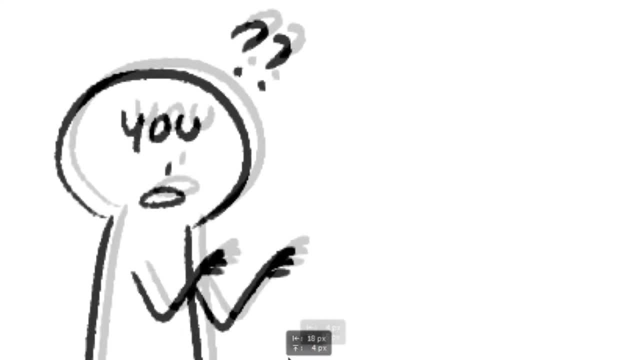 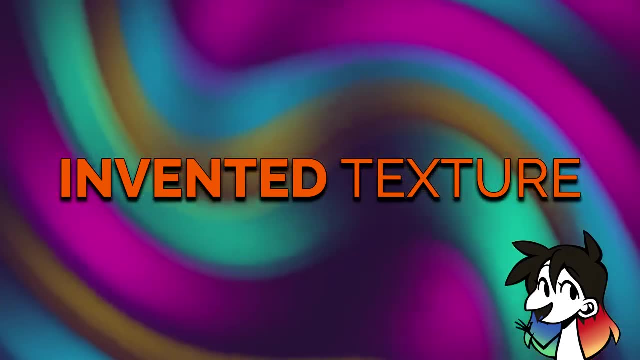 Jesse, you've basically said texture is either real or not real. What else is there? Don't worry, there's more. It just gets a little weirder from here on out. Invented texture is a texture that doesn't actually exist and is created by the artist. So let me draw a bunny. What texture? 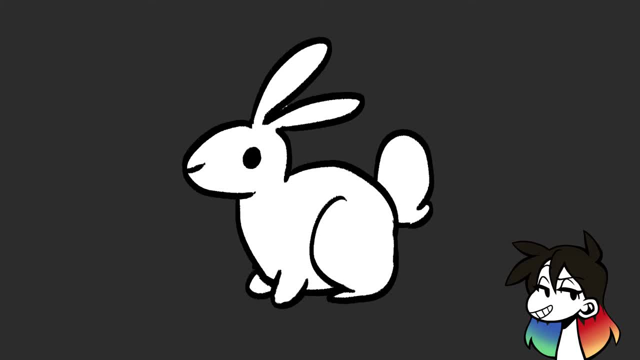 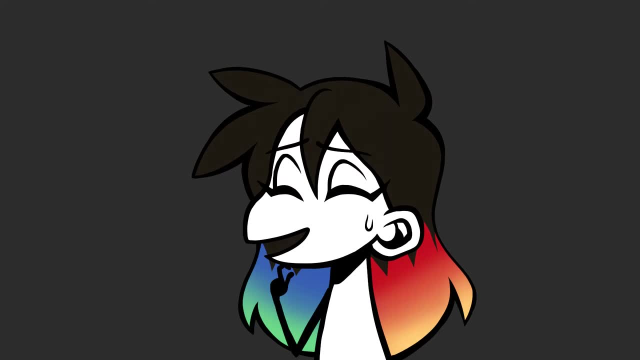 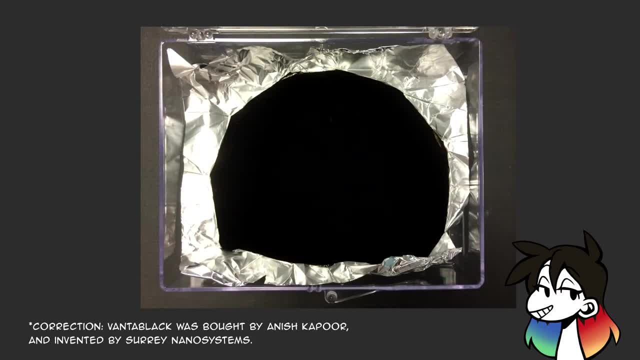 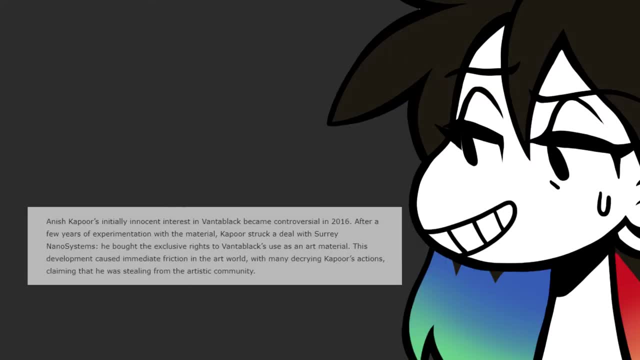 Vantablack was deemed the blackest black in the world because it was able to absorb 99% of the light around it. It looks like you're staring into a void. There was a lot of controversy around the medium, but even so, you have to admit that that's pretty cool. 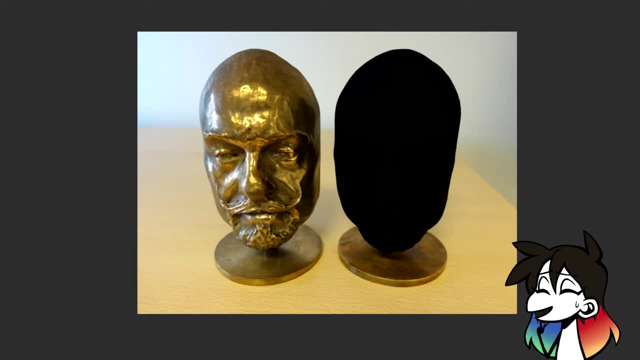 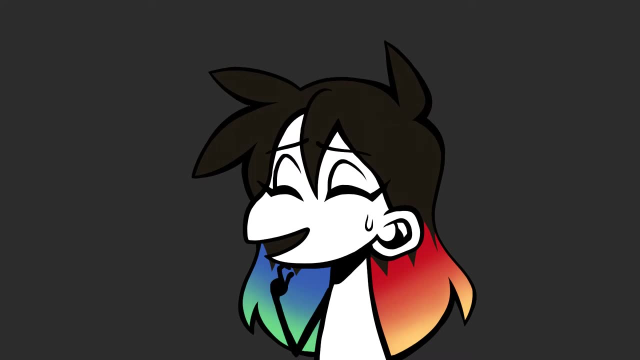 Notice, however, that it's a man-made texture or lack of texture, and you'll never see it anywhere in the wild or in any normal circumstance. That's invented texture. There's one more type of texture to explain, and this one might be the strangest. Abstract texture is when existing textures are. 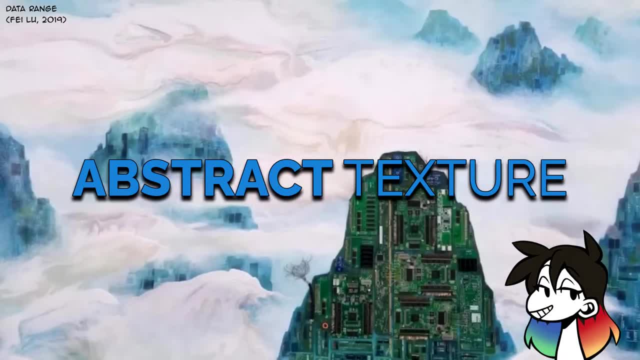 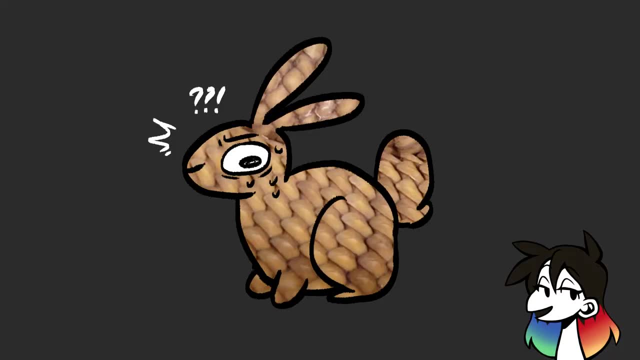 used out of context in order to portray a new idea or create new emotions. This is often known as juxtaposition. So let's take that bunny again, but instead of fur I'll give it scales. That's abstract texture, putting other textures where they don't technically belong. Take object Le. 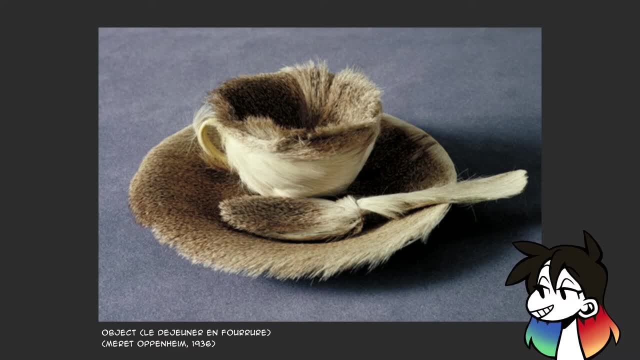 Dijonais Inférieur by Murray Oppenheim. I don't think I need to tell you that cups, spoons and plates aren't supposed to be fuzzy, but I'll point it out anyway for the sake of the video. This piece in particular was meant to show how nice fur is to touch, but the one place we don't 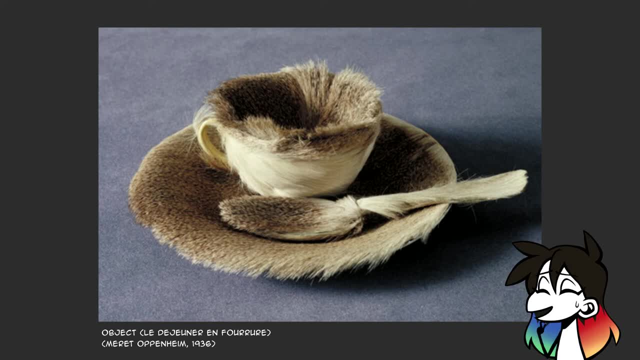 like to have. fur is in our mouths And you know we kind of have to put cups and spoons in our mouths Because this fur isn't where it's supposed to be. it's a form of abstract texture. This technique feels very surrealist. 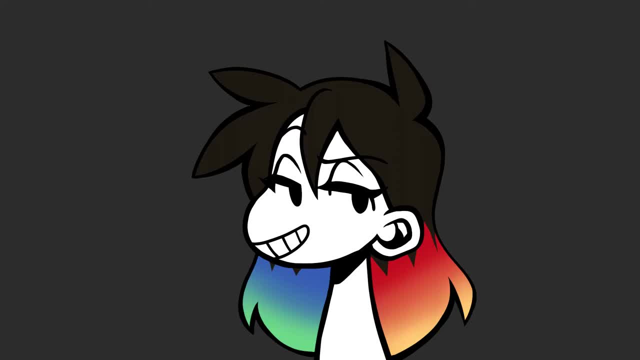 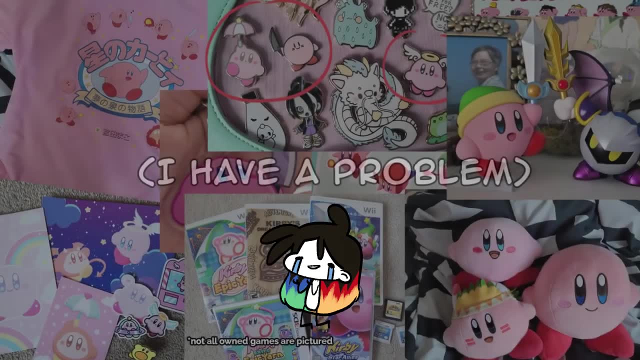 though you tell me, This doesn't seem like something I should apply to my current artwork. Au contraire, my friend Kirby's Epic Yarn is actually another example of abstract texture. Yes, finally a video where I can talk about Kirby Everything, and I mean everything in. 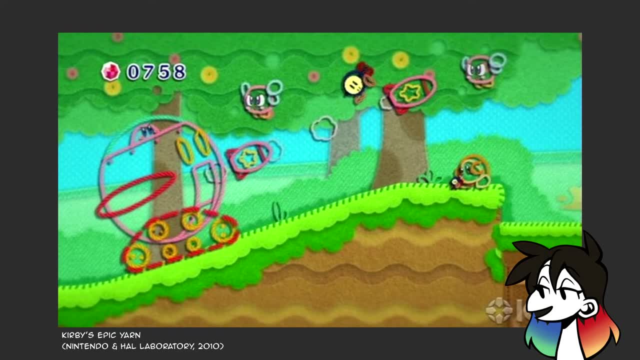 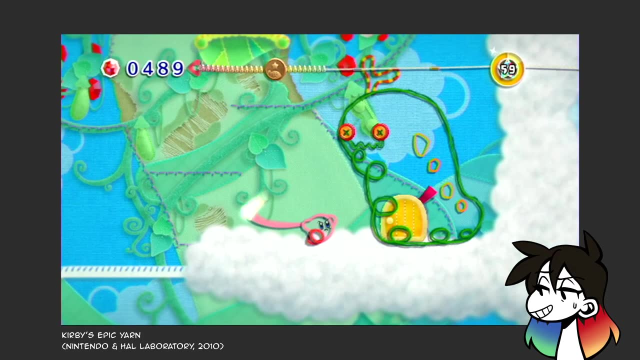 this game is made of fabric or yarn: The trees, rocks, ice, food, characters- it's all made of textiles and string and everything sewing-related you can think of. Of course, our trees aren't made of fabrics and buttons and our clouds aren't made of stuffing. 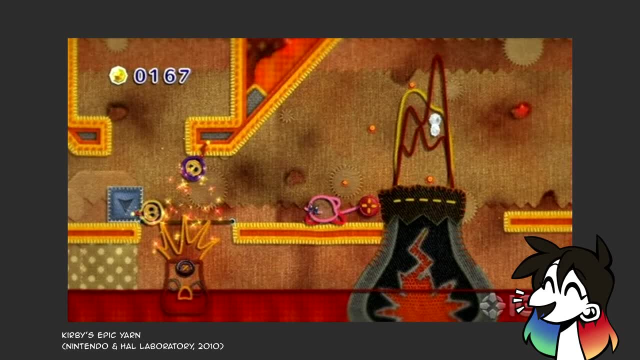 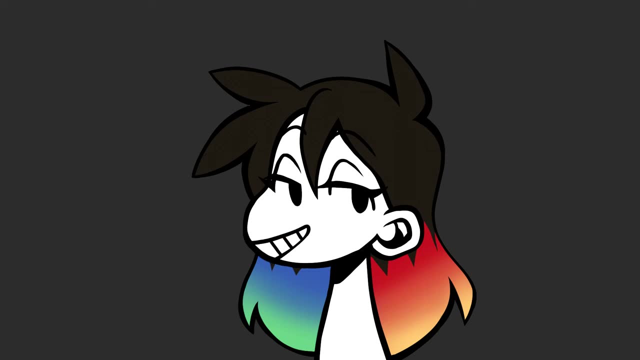 but it gives a whole new feeling to every bit of the environment. You'd never think a volcano would look so huggable. Playing around with abstract texture is a fun way to add new feelings to your artwork and can give it that extra push to make it something truly unique. 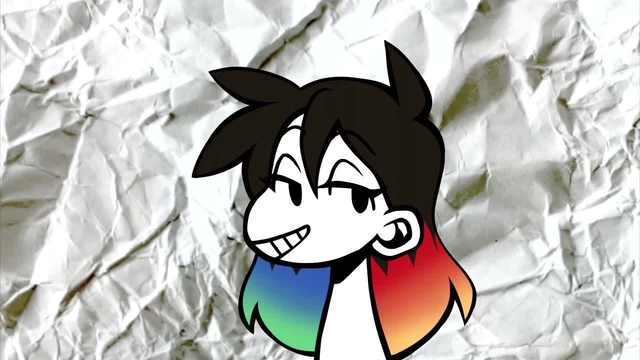 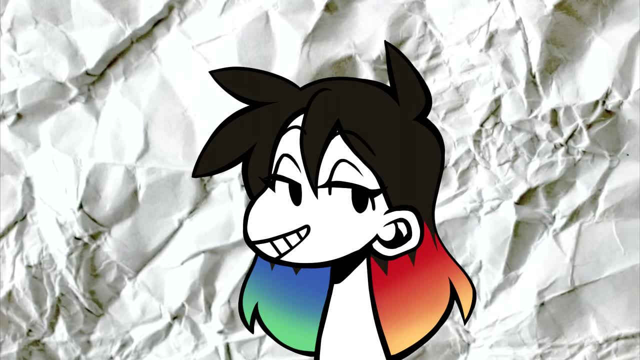 Texture, in terms of its concept, is pretty simple but also really flexible. It's either there, not there, looks like the actual subject, or doesn't look like the actual subject. But that flexibility means that there's so much you can do with it, Especially with stylized work, you can. 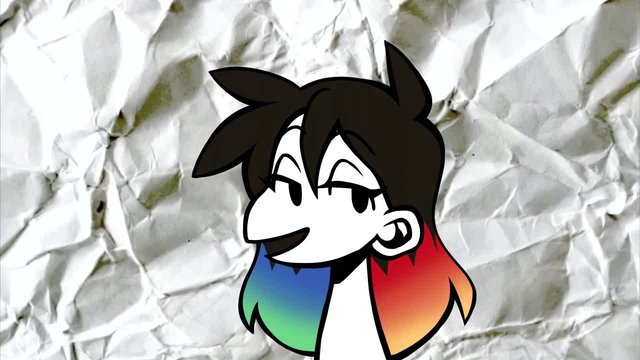 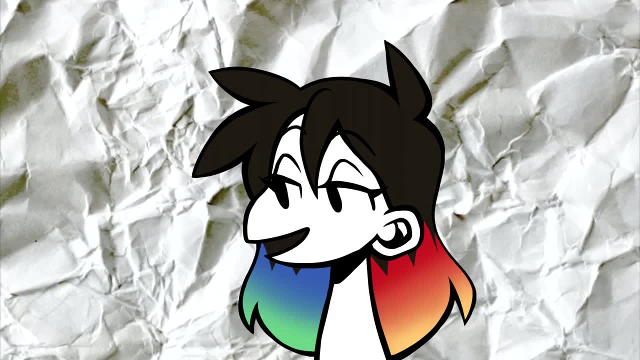 mess around with how you present your textures And who knows, if you mess around enough, maybe you can create a whole new style if you experiment a lot. But the best thing about texture is that as long as you let your intended style shine through, you'll always be creating great works of. 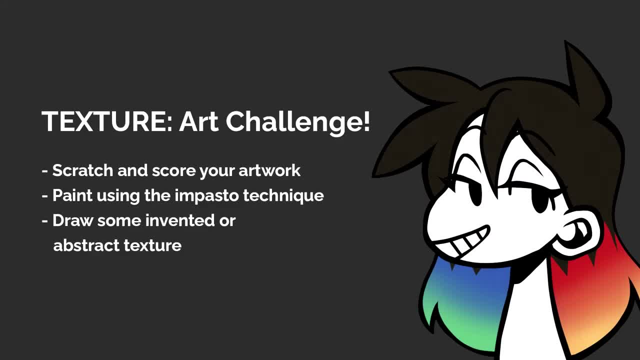 art For your next piece. think about how you can utilize texture in different ways. Try adding different kinds of actual textures with different techniques. Scratch up the paint score and pinch your clay. see what you can make your artwork feel like If you have some paint lying around. 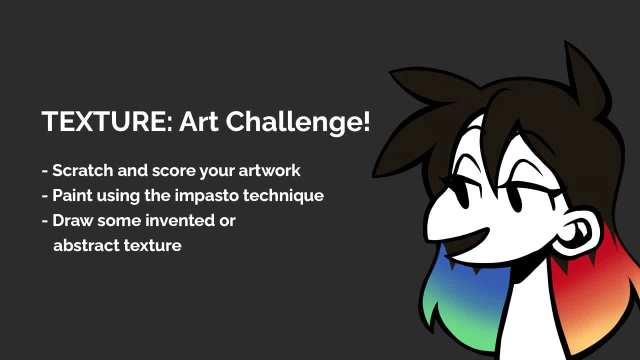 try to paint something with an impasto technique. Or, if you're not much of a painter, try to draw something with either invented or abstract texture. See if you can give your artwork a different feeling by switching up its textures. If you're a teacher, we have worksheets on the topic. 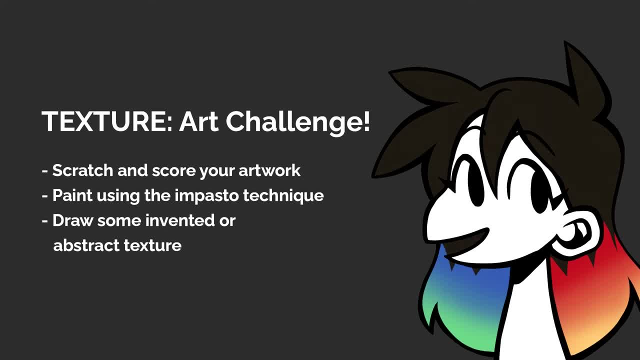 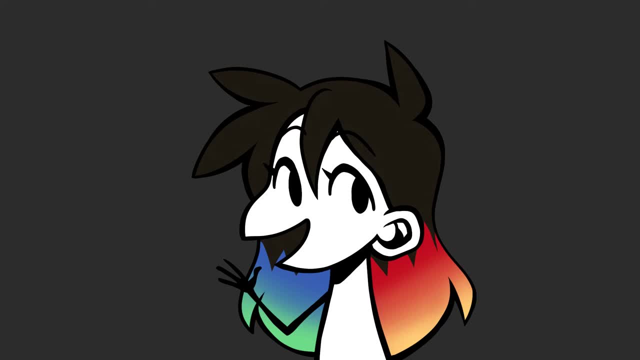 which you can find on our website, along with other art resources for your classroom. link down below. If you liked what you saw, be sure to leave a like on this video. comment down below to let us know what you'd like to see us do next and hit subscribe so you never miss an upload. Join our. 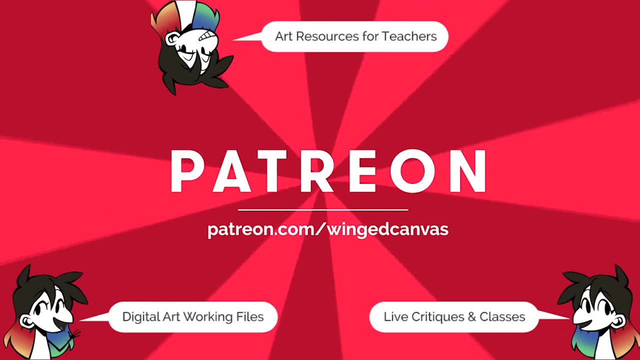 little art community with the links down below and support us on Patreon to get sneak peeks, critiques and teaching resources. If you enjoyed this video, here's a couple other videos you can check out next.